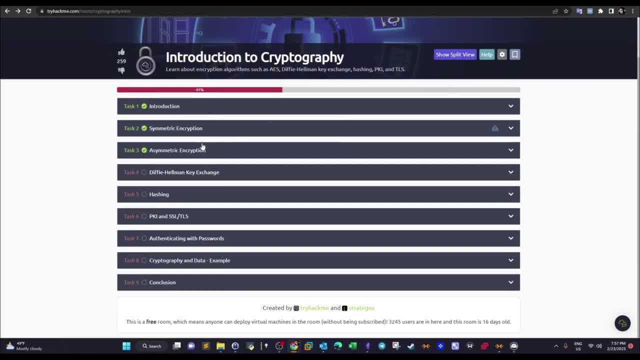 tackle the use of the tools or symmetric and asymmetric encryption tools, how mainly there are two. there are many tools, but mainly we're going to discuss two tools: open ssl and the gpg project. so these two tools can be used to encrypt and decrypt using asymmetric, asymmetric and. 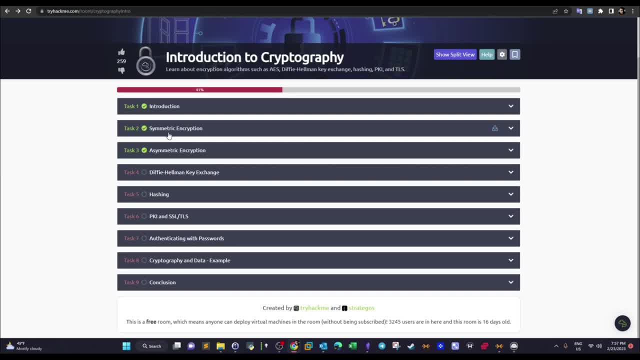 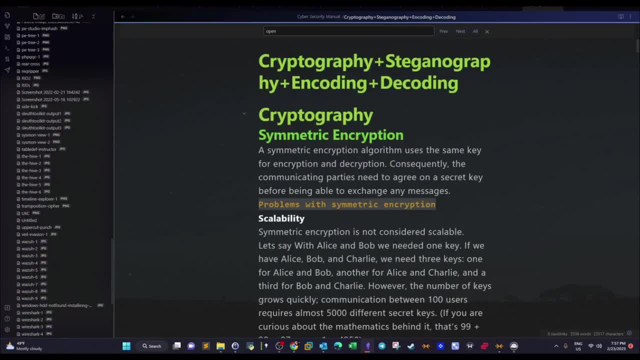 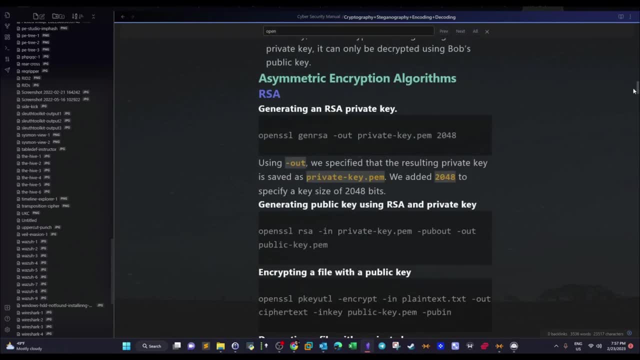 symmetry encryption. but before using these tools, let's first give you an intro. now, basically what i have done. as you know, guys, members of the channel, i have added some updates on the cryptography notes covering the tools that are used in the current scenario. okay, we're going to use the. 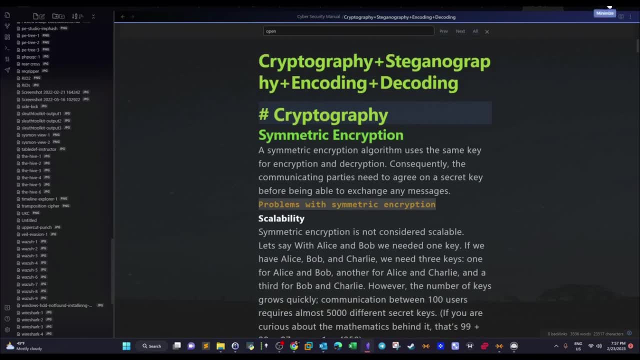 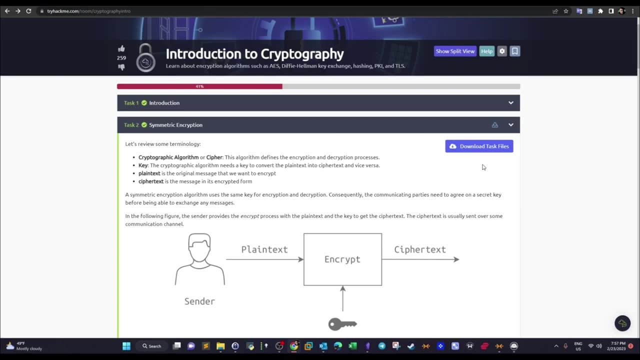 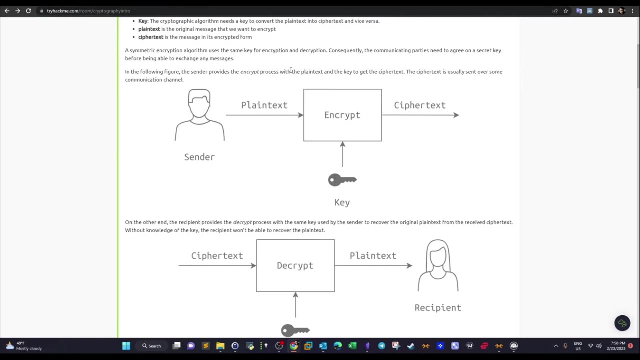 notes here to solve the tasks. but before using the notes, let's go back and give you a little bit of introduction on symmetry encryption. so, as you know, guys, in a nutshell, if you don't want to read all of that in a nutshell, in the symmetric cryptography or some other encryption, we have center and we have receiver. 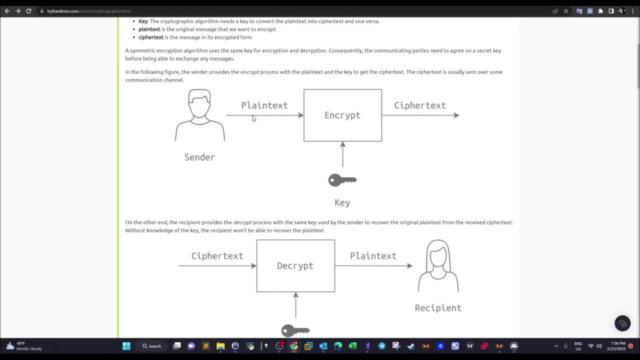 recipient. so basically the plain text is the piece of information that is to be encrypted. we encrypt the plain text or the secret with a key. the key is known to the sender and the recipient is a secret key. so basically both of these parties know the key but, of course, outside. 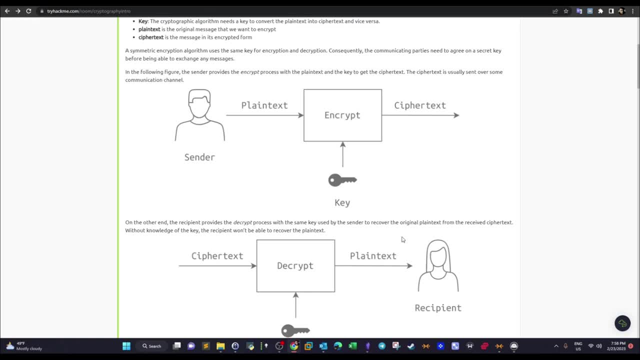 parties, those who are actually not intended to view the plain text message, don't have the key. so with the simple key, with the same key, we encrypt the plain text or the encrypt the message and at the same time we decrypt the ciphertext. the plain text is the message before. 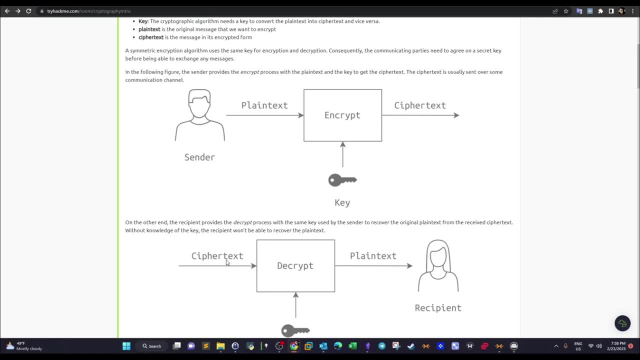 encryption, the ciphertext is the message. after encryption, the plain text is encrypted with the key and the same key is used by the recipient to decrypt the ciphertext. in a nutshell, the problem with symmetric encryption is that symmetry encryption is not scalable. so if we have, for example, um 200- uh people, right, 200 persons, i want to communicate each one of these. they want key and 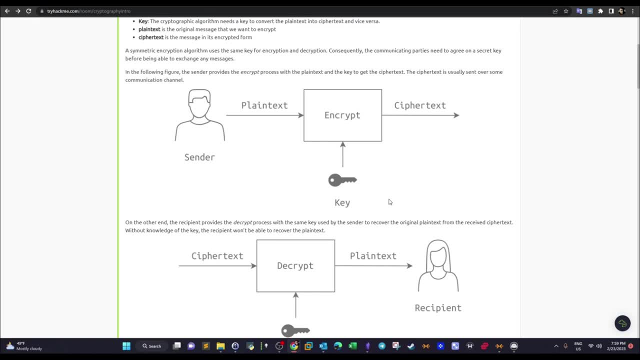 the options are limitless. so if you have 200 mainly we're gonna need like over 2 000- 3 000 keys. if one of these keys are is lost, we're going to renew the whole system and generate a new 2000 or 3000 keys. 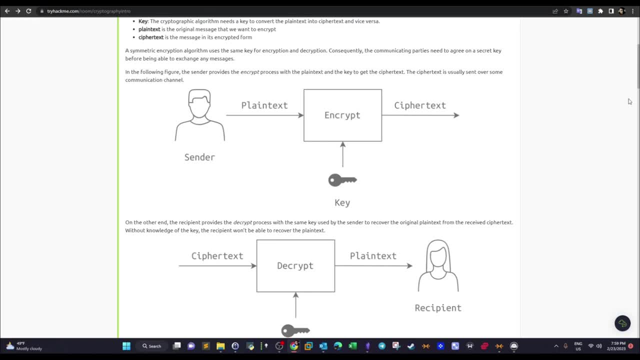 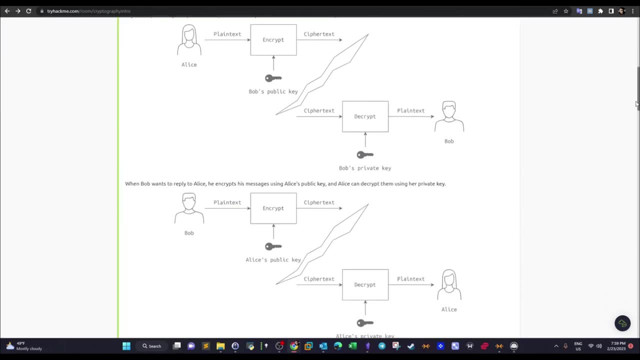 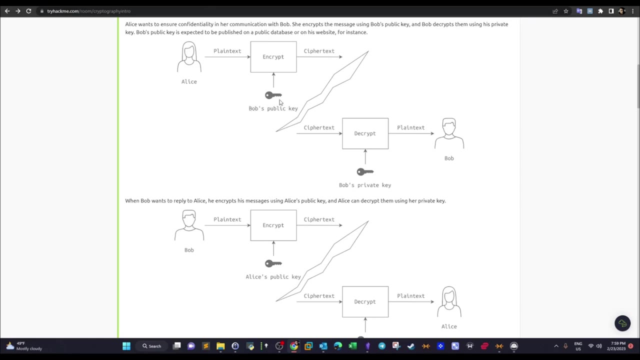 so it's not scalable, but it is fast way of encryption. now, asymmetry encryption is actually kind of slower than symmetry encryption. why? because in symmetry encryption we have two keys. we have four keys in general, so we have four keys. so basically what happens here is that. 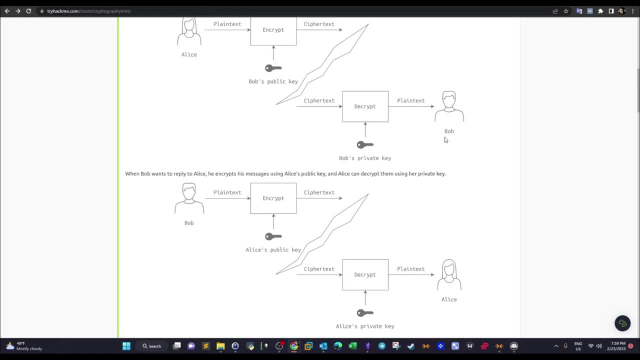 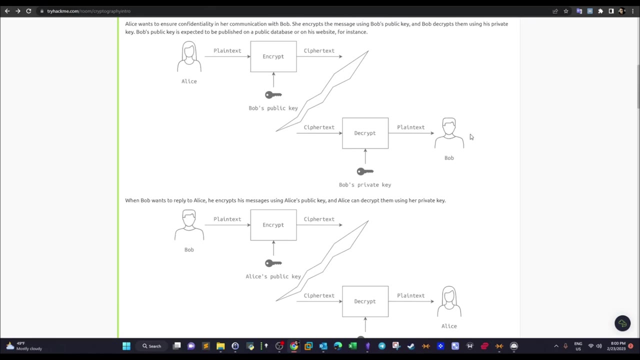 say we have alice and we have bob, like always, right the same example in all that, in all scenarios, alice and bob, they want to communicate. so alice has a piece of uh text or information she wants to encrypt. so basically what she's going to do, she will use bob public key. okay, so using bob. 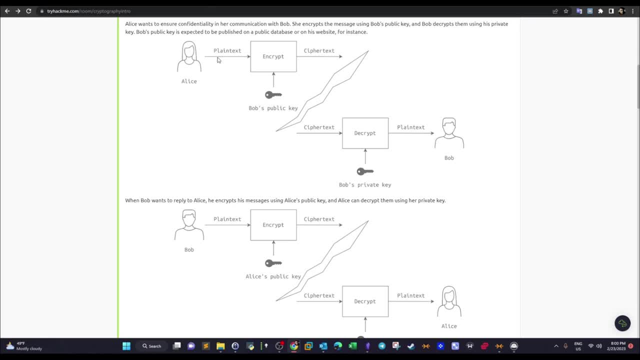 public key, she will encrypt the plain text message. the plain text method becomes a ciphertext, as you can see here. so bob's public key is used to encrypt the main message that's going to be sent by alice. now bob will receive a ciphertext, as you can see, created by alice in order for bob to decrypt the. 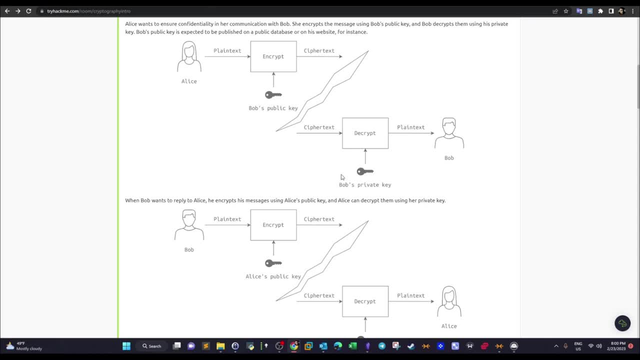 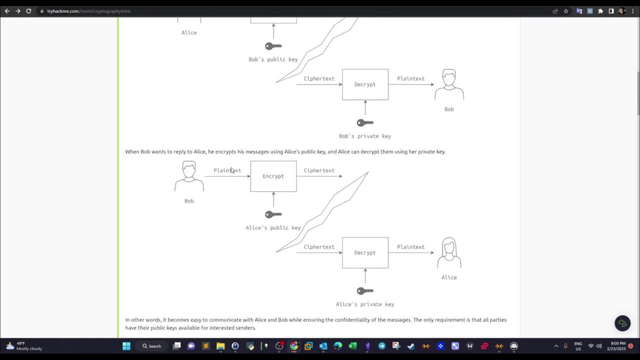 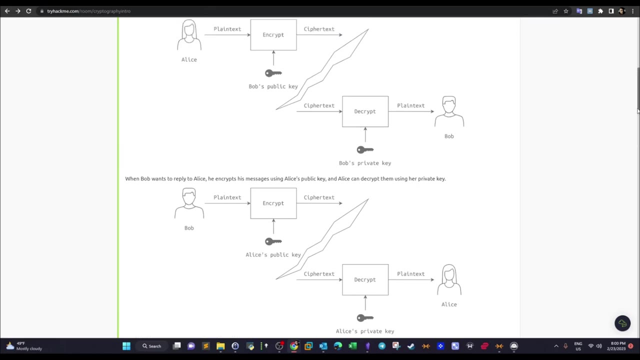 ciphertext into plain text. he's going to use his private key right and vice versa. when bob wants to send a piece of sensitive information to alice, he's going to need alice public key here. so, as you can see, guys, there is a pattern to the process. the public key of the recipient is used to encrypt. 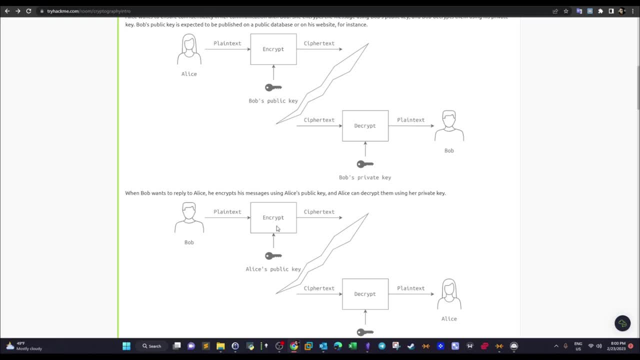 the message, the public key of the recipient in both cases, as you can see here, and the private cube. the recipient is used at the same time to decrypt the message. but the thing is, the private key of pop and the private key of alice are sensitive and private. no one knows about them only. 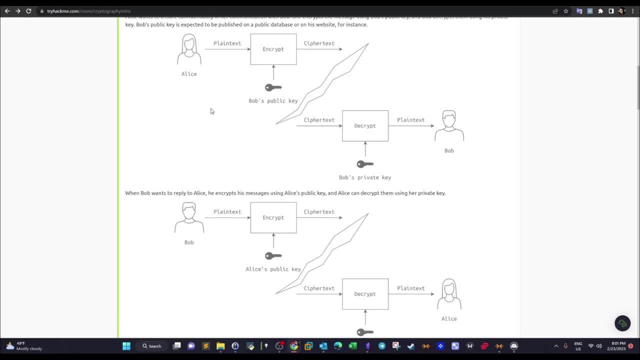 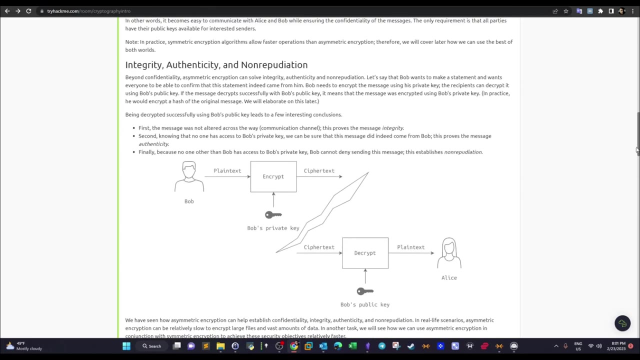 the public key is known. actually, the thing with pop, with the public cryptography as they call it, or asymmetric encryption, is that it's slower than the uh symmetry encryption, but it is scalable and more flexible and more secure. so basically, that is a nutshell of both symmetric and asymmetric. 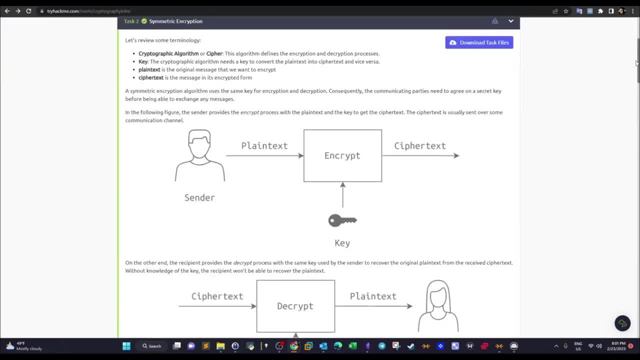 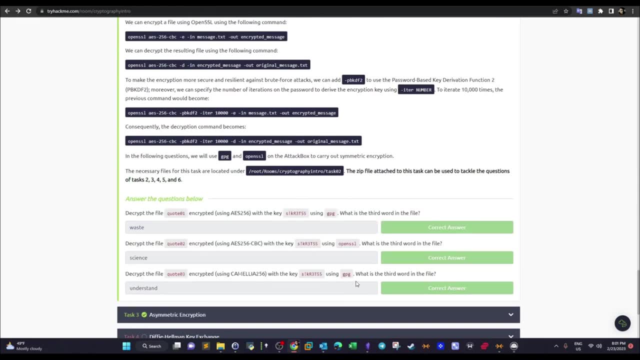 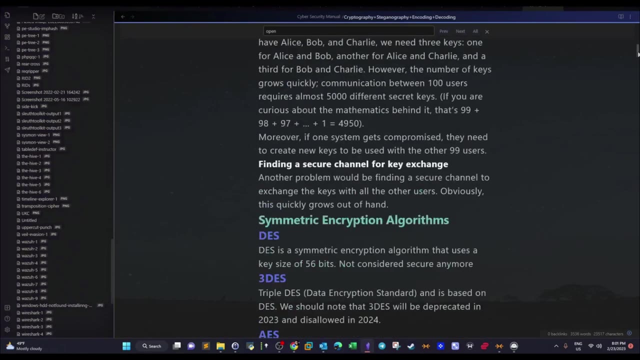 encryption. now, more important, let's discuss the tools in this task. so basically, here we have three questions now in the three questions, we're going to talk about how to encrypt and decrypt files- okay, using symmetric encryption. now, in symmetry encryption, we have two tools we can use. so symmetry encryption tools are: gnu privacy guard. 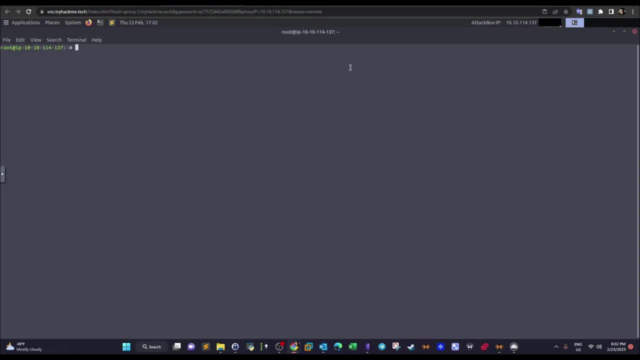 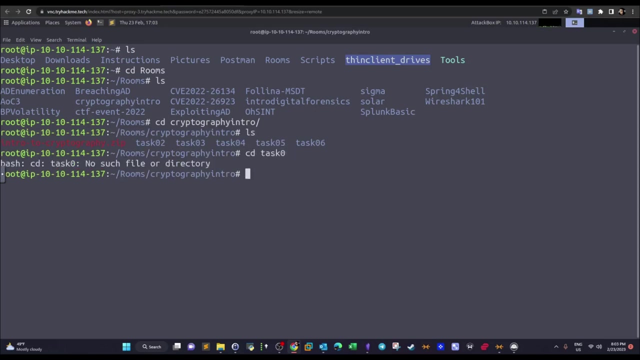 and open ssl project. so let's hop into the attacker machine here, dls. and of course you want the phone bigger. i'm going to do that for you. so cd runes and the files of this task are located under crypto intro. okay. cd task02- okay. so, as you can see, we have a ciphertext with the extension gpg and we have another. 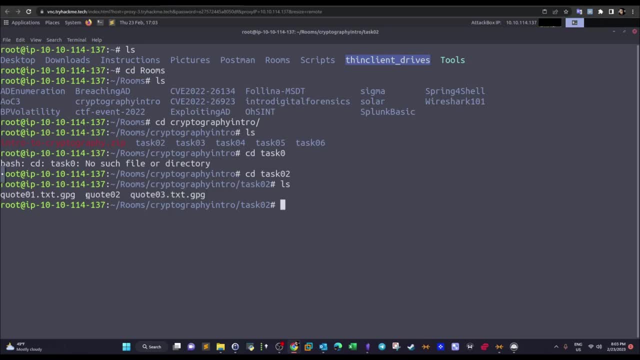 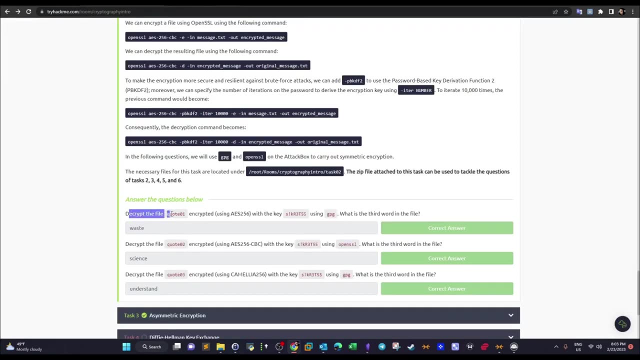 ciphertext with the extension gpg as well, but ciphertext code02 doesn't have this extension. so what we're going to do? the first question: decrypt the code01 encrypted using as 256. so basically, as256 is a symmetric encryption algorithm. i have divided the encryption algorithms here. 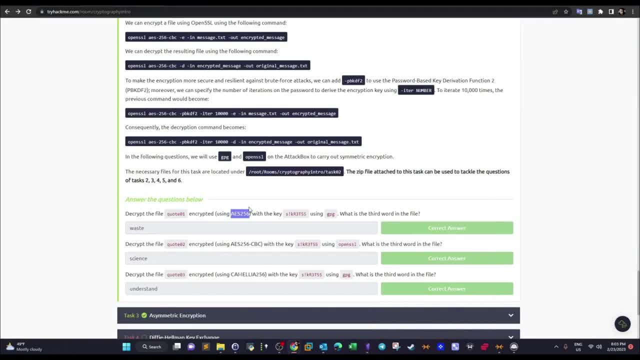 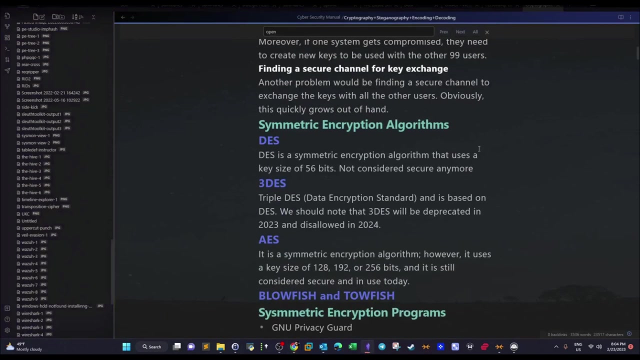 ds, 3ds as bluefish and towfish, basically, essentially here. as you can see, code01 is an encrypted ciphertext. okay, using the aes algorithm, and this is the key that has been used to encrypt the ciphertext. what we're going to do? we're going to need to decrypt that ciphertext using the gpg. okay, let's go here and find what. 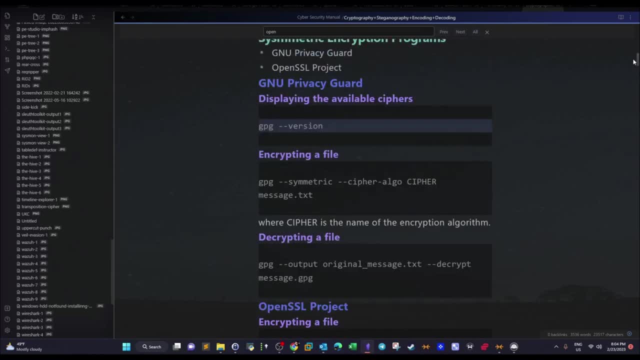 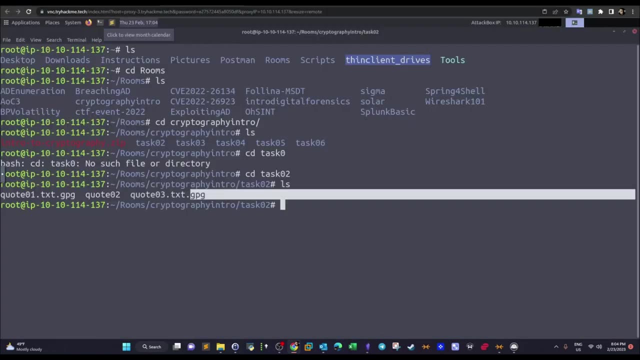 we're going to do okay. so this is a way to encrypt and this is the way to decrypt. so let's copy the command and paste it here. i'm going to change a couple parameters here, so basically the original message. since we are decrypting code01, i'm going to name it code01.text and we're going to give the input. 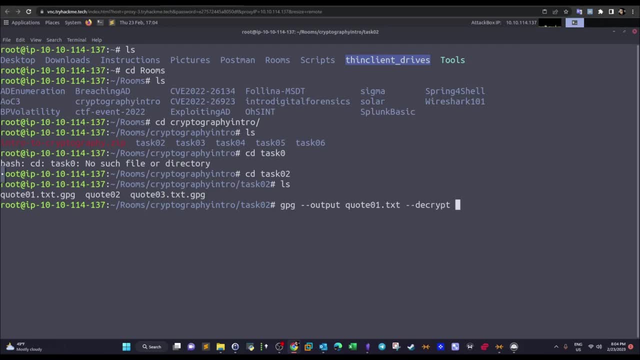 which is the ciphertext. as you can see, it recognized the algorithm aes256 and now it is prompting us to decrypt the code for the password or the key. so we copy the key here and paste it in. let's get code01. okay, so that is the main plain text. 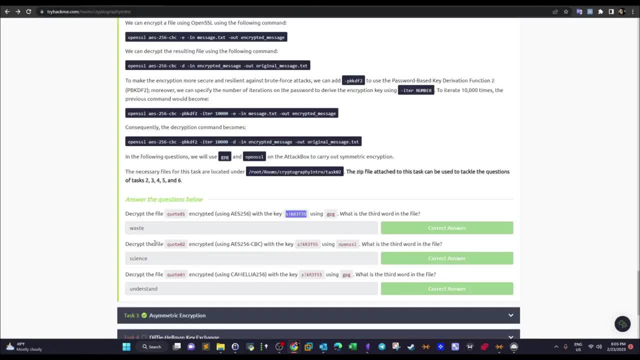 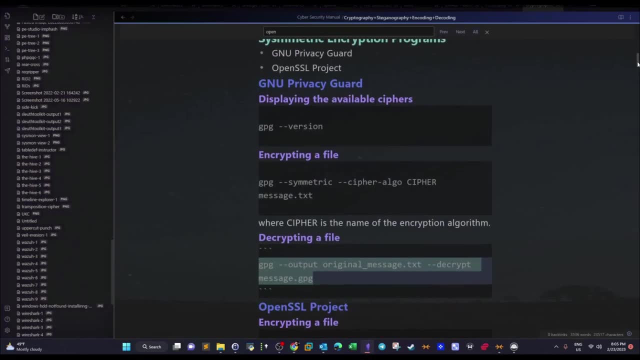 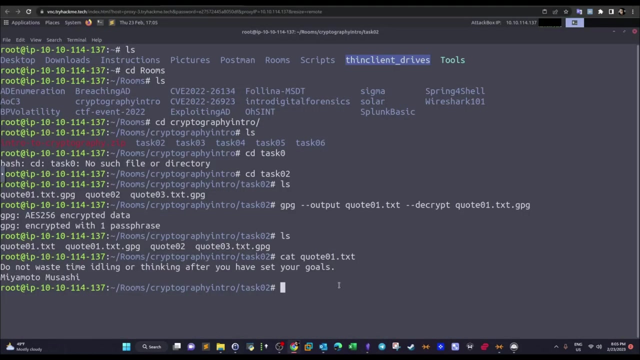 and the answer to the question is the third word, which is waste. next question: decrypt the ciphertext code02, which was encrypted using aes256 cpc, along with the key, using open ssl this time. so let me go to open ssl and see how we can decipher a ciphertext. that's the command heading back here. 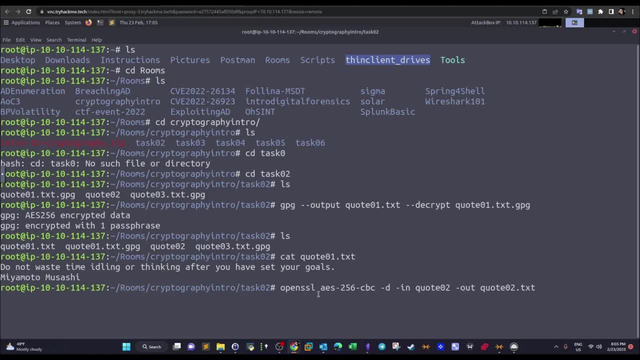 okay, we're going to change on all of that. so basically, that's how we specify the algorithm. dash d for decrypt. dash in is the ciphertext which is already specified in the command, and that's out specifies the name of the file that will contain the plain text or the deciphered ciphertext. 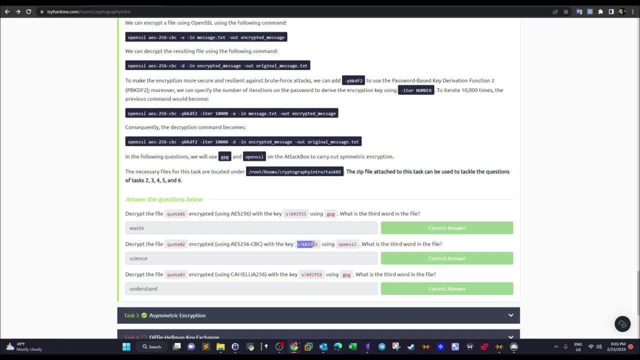 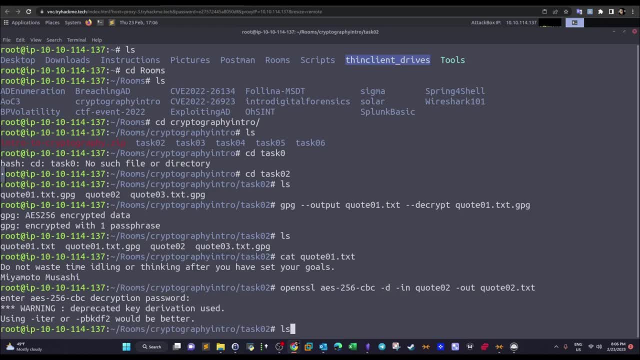 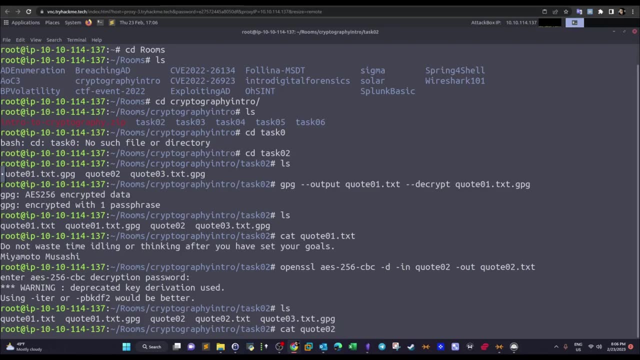 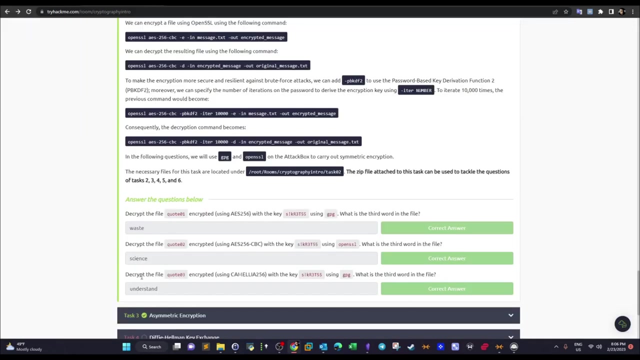 and here it is prompting us for the password or the key we're going to copy that it's already given. get code. all right, it's true science of martial arts. decrypt the file code03 encrypted using camilla a256 or camilla256 with the key using gpg. back with 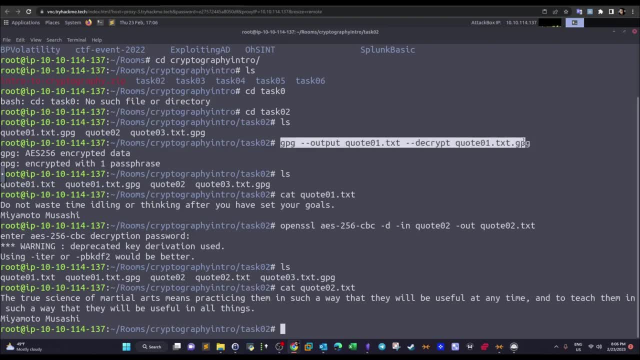 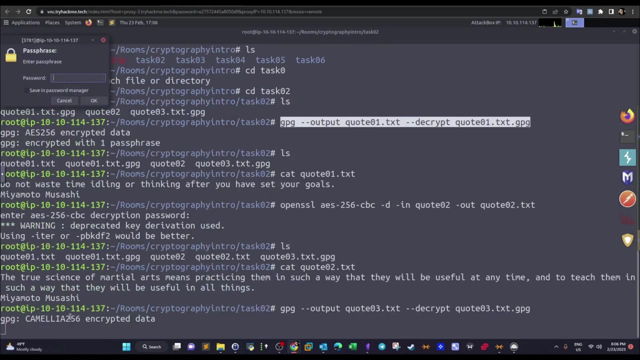 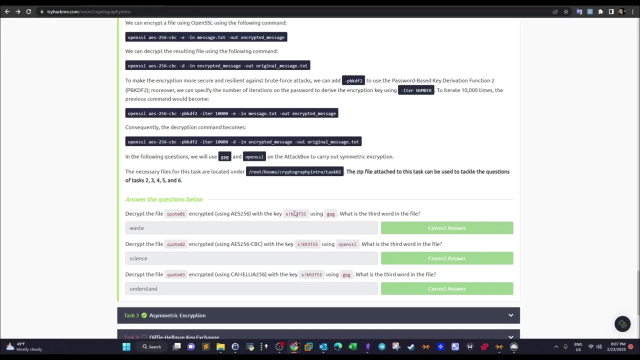 the same command. we're going to take this one and specify code03.text as the output, and the input will be 0.255.7. simple, as you can see, the algorithm has already been recognized and we all need to paste in the key to solve the challenge, as you can see. as you can see, guys, so far, as long as the key is known. 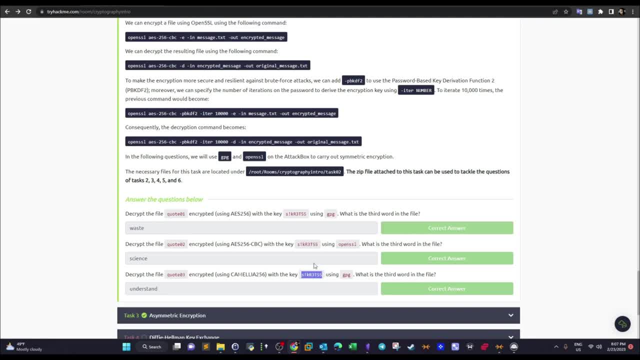 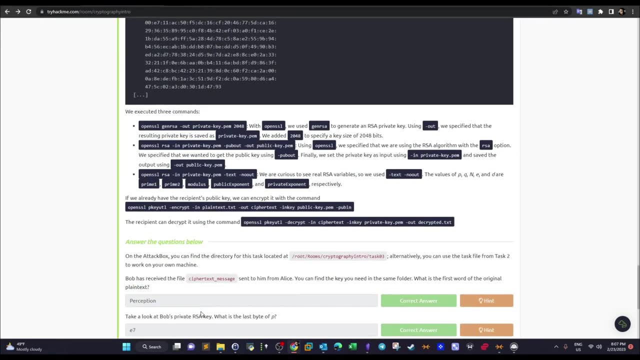 the operation is easy. but once the key is absent, right crack the key. so basically that's what we call the secret key in the symmetry encryption. that's the key used for encryption and decryption at the same time or simultaneously in symmetry encryption. now let's go ahead over asymmetric encryption challenges and we're going to 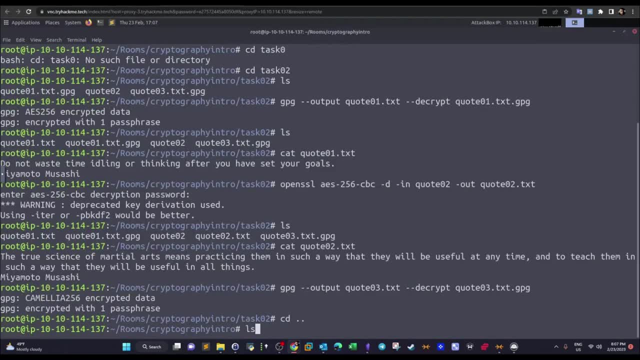 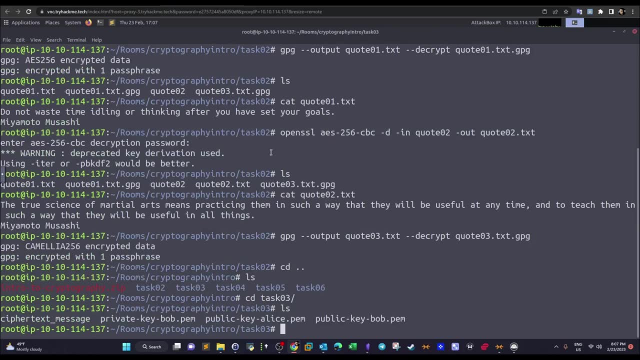 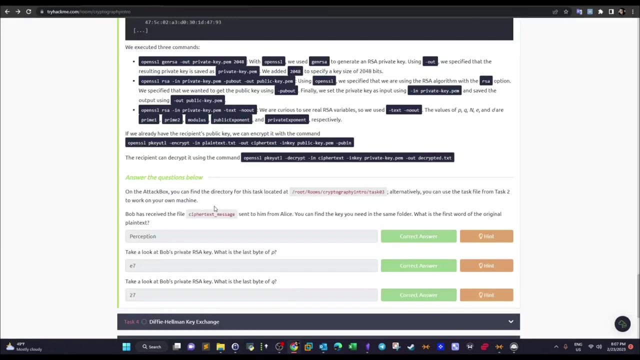 talk about it. so cd back, cd, task 03. okay, as you can see, we have these pieces of information. we have the cipher text, the private key of bob, the public key of alice and the public key of bob. let's go and understand the scenario before going to the scenario. guys, as you can see, there's a mention of rsa here. rsa is 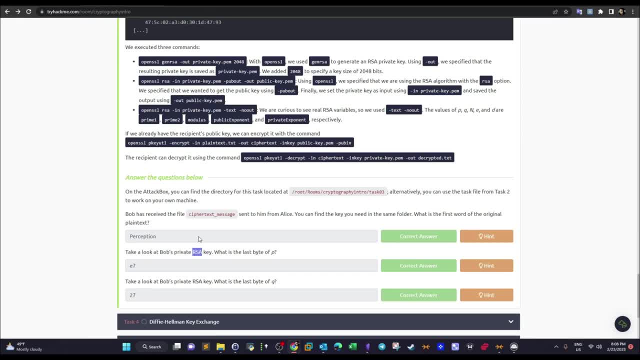 the public key algorithm, public encryption algorithm. okay, and there are many tools used to encrypt and decrypt you using rsa, especially rsa ctf tool that if you are a ctf solver, you might have come across this tool before. so let's talk about the scenario here. so bob has received the file. cipher text. 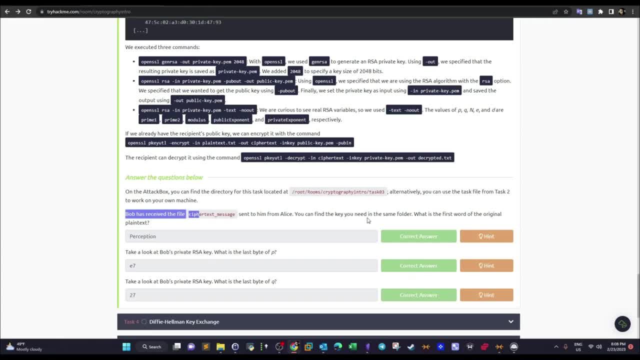 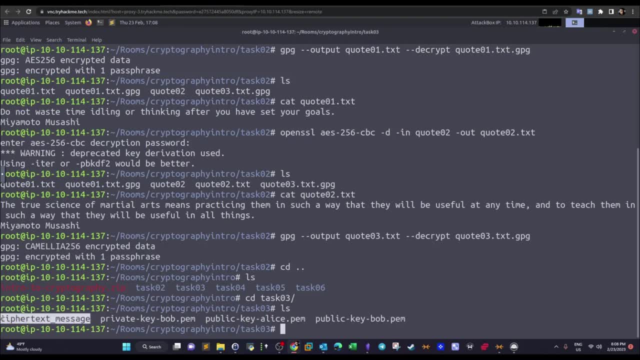 message sent to him from alice. you can find the key you need in the same folder. what is the first word of the original plain text? so bob has received this cipher text? okay, most probably, oh, not most probably, it's definitely. the cipher text has been encrypted by alice. okay, but by what? by using the public key of bob. so bob will need to decrypt the. 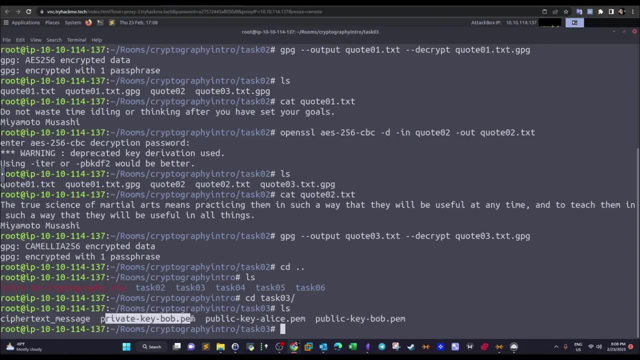 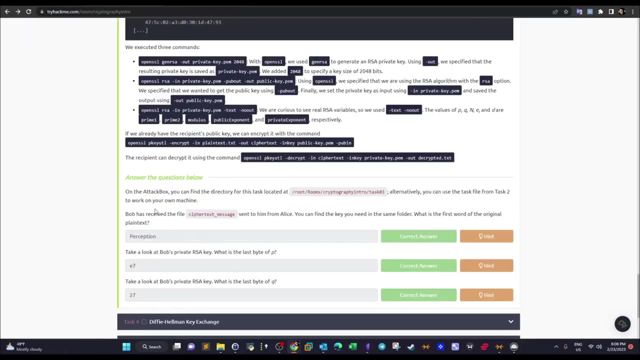 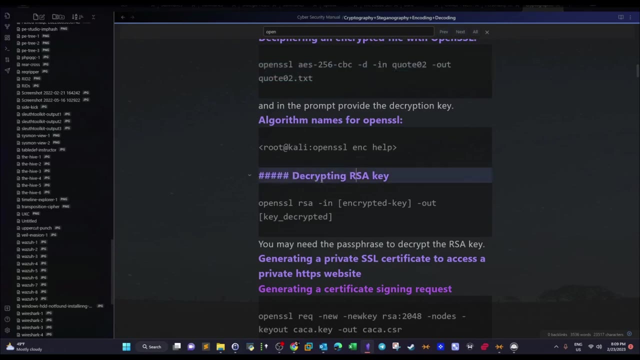 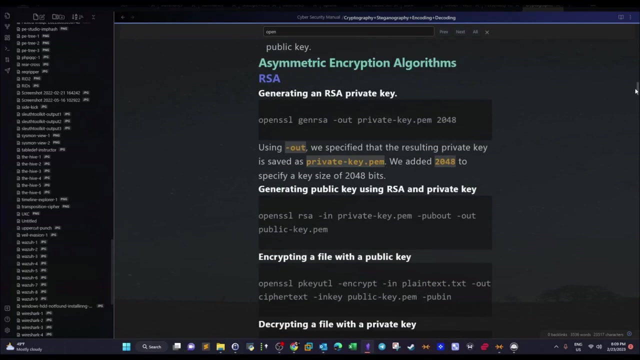 cipher text message using his private key. he is the recipient of the cipher text, so he's going to use his own private key to decrypt the message. okay, so how to do that? we're going to find the notes. okay, decrypting rsa key. okay, so with open ssl, we can decrypt a file with a private key. this is the command. 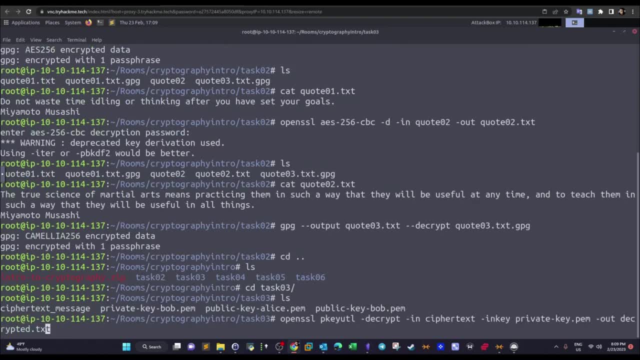 i'm going to paste this here. all right, let's see. so: open ssl dash decrypt and the cipher text is here. so we're going to specify a cipher text. now. the key that will be used as an input is bob private key. so we specify bob private key here. 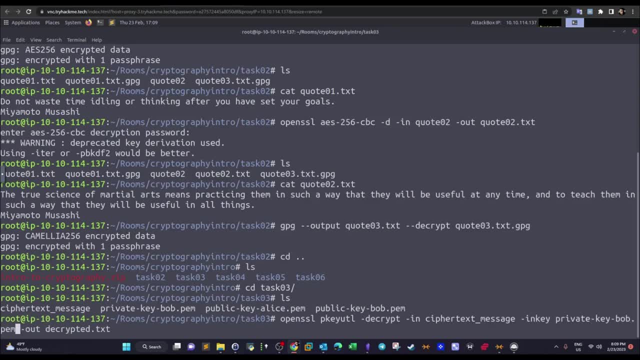 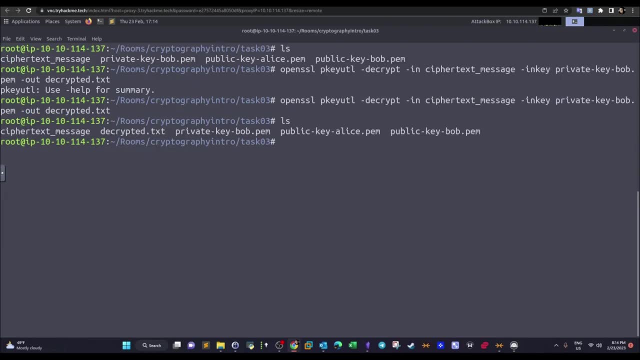 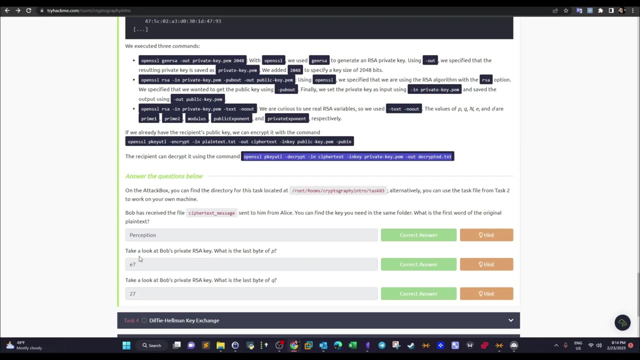 private key bob, and here we can select the name of the file that will contain the decrypted output. okay, cats decrypted. and this is the cipher text with the plain text. take a look at bob's private rsa key. what's the last byte of p? now? basically, guys. 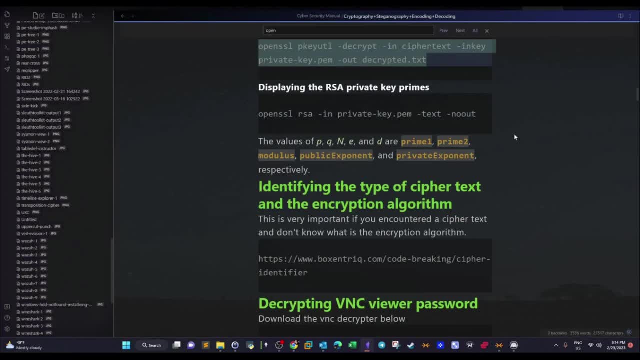 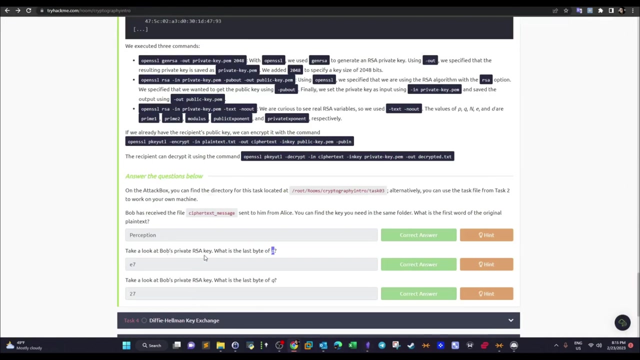 let me go back here. so p, q, n, e and d are important factors used in rsa encryption. so basically, normally when we do rsa encryption or decryption, we aim to find the value of these. okay, so the question here: and these values are stored in the private key. so the question here is: take a look at bob's private key. 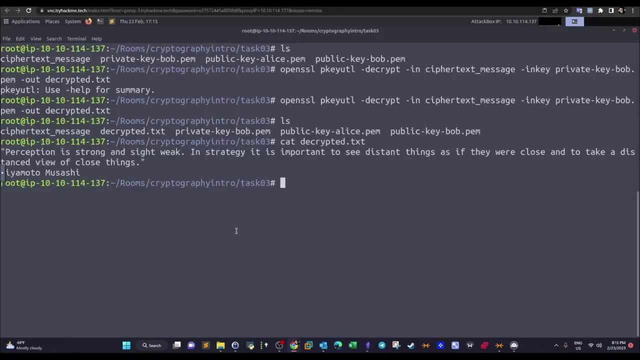 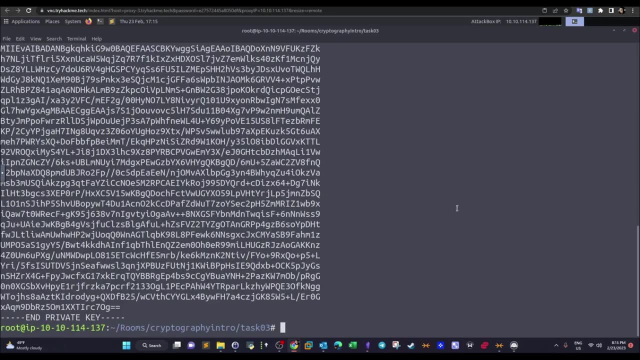 rsa key, what's the last byte of p? so if we ls and cat private key bar, this is the private key. but this is not a way to view the private key right and or to extract these parameters. so what we have to do, we have to use open ssl. so how to do that? 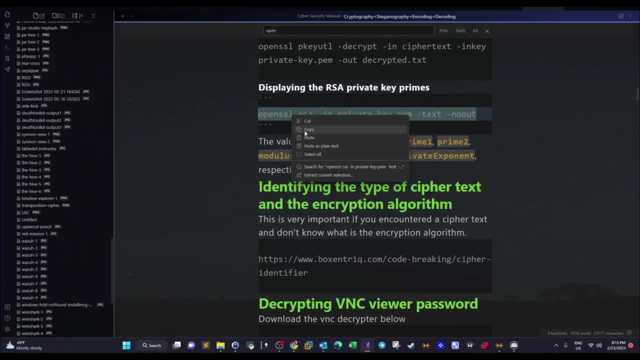 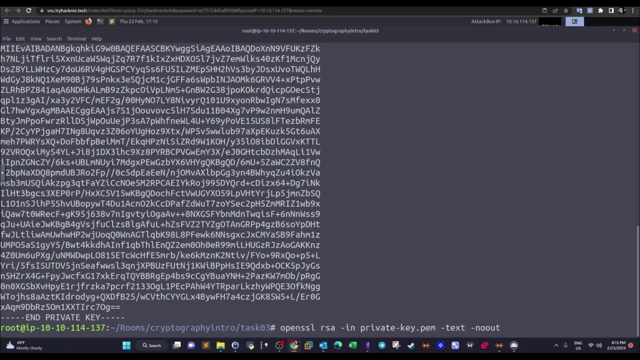 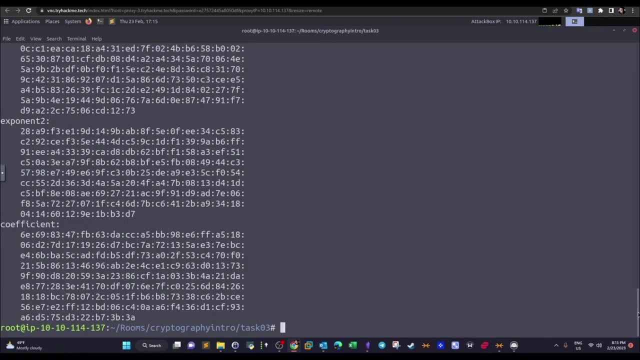 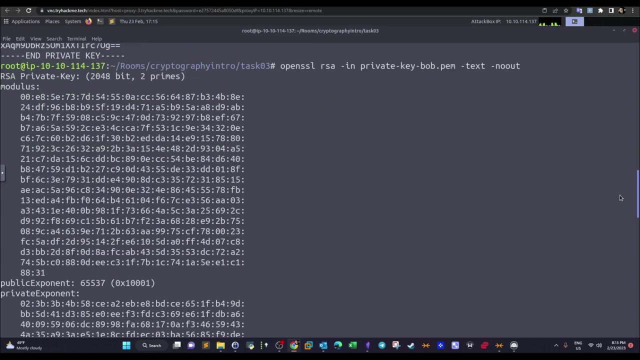 we're going to use this command to display, to display the key primes. so we call them the key primes and here we use the name finally, above private key. okay, as you can see, we were able to display in hexadecimal format, of course, the values of the key primes. okay, so prime one is p. 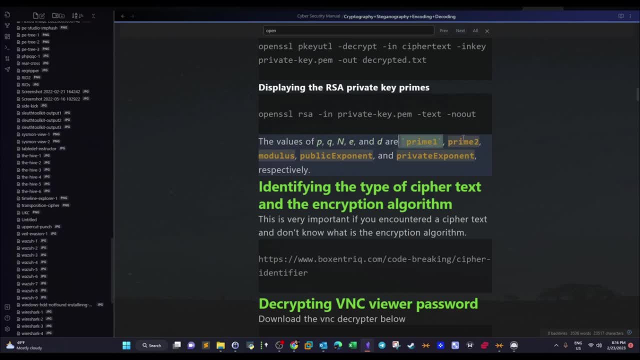 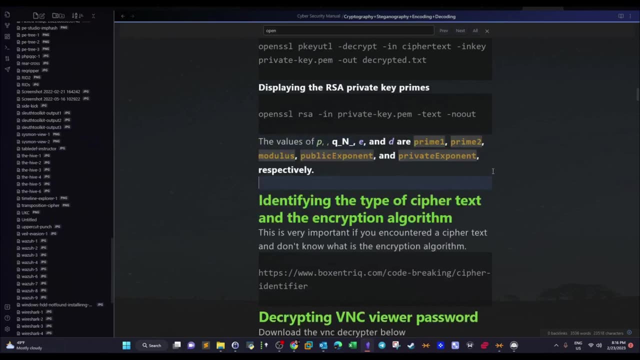 as you can see here, p is prime one. prime two is q and is modulus. oops, what happened man? okay, and i have no idea what happened here. p, q, what? i'm gonna fix this later. p queue n, e and d: as you can see, prime one corresponding to prime. 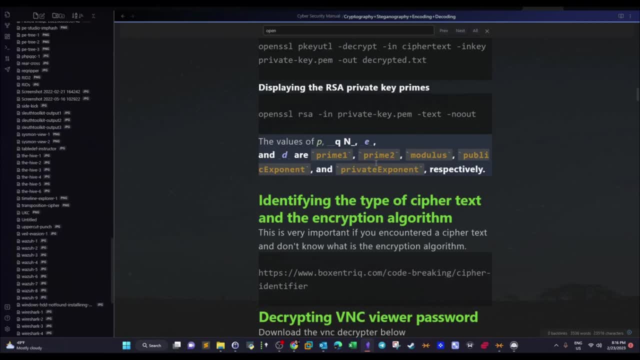 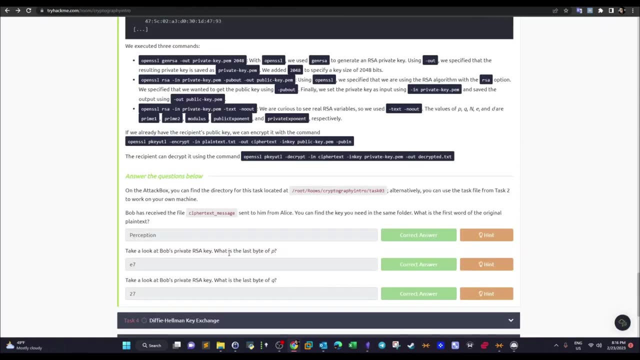 one and prime two: modulus: public exponent and private expense respectively. so this that's how we match them. so prime one: the question is what is the last bite of p which happened here in the private way? общ evangelical common 3, prime 1 is e7. that's the last byte. and what's the last byte of q? q is prime 2. 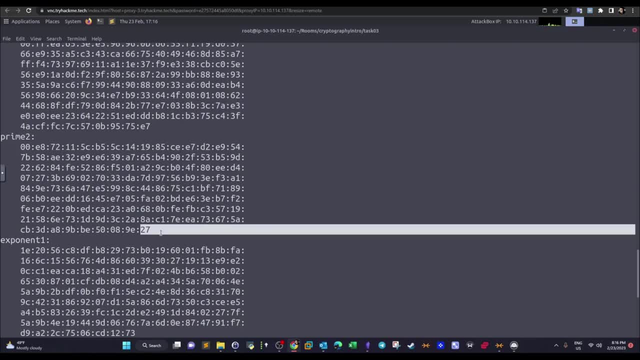 and this is the last byte of q- you're going to need to understand the use of both these tools: open ssl and the gnu project to decrypt and decrypt using both symmetric and asymmetric encryption. guys, when you are dealing with ctf challenges or maybe cryptographic challenges, sometimes you may need 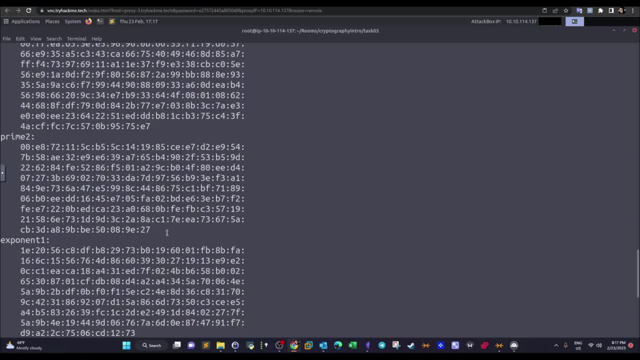 that while doing pen testing, if you have come across some sort of rsa private key, you want to decrypt it. you will need to use open his sale. you need to use the to understand the role of these key primes and the factorization and how to find the values of each one of them. 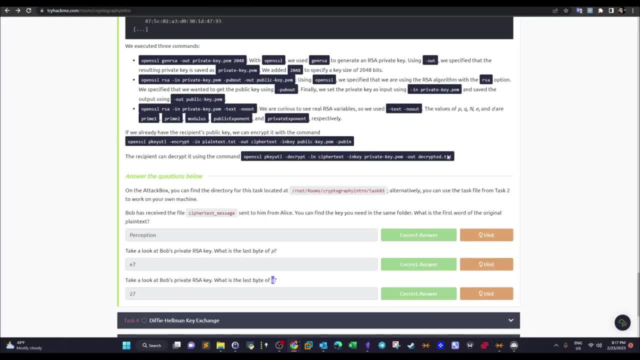 so, basically, guys, that that's. that was it. i hope you like that, and later we will carry over the rest of the cryptographic tasks and see you in the next video. 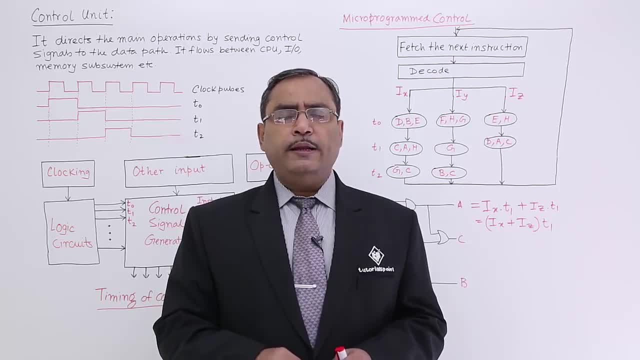 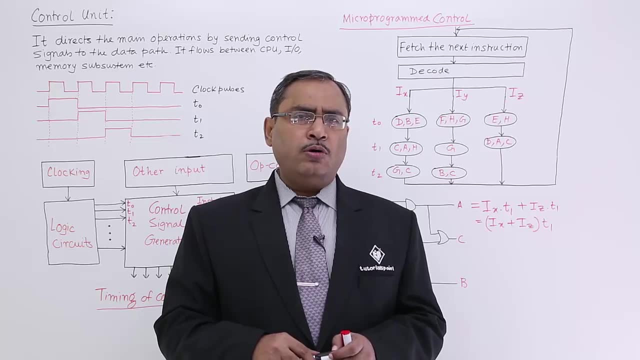 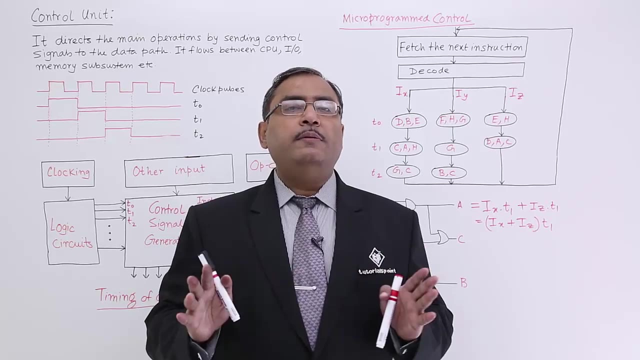 Now in this session we are going to discuss control unit. That is a very important topic for your semester exams and for the GATE exams also. So what is a control unit? Control unit is nothing but one unit where it will generate control signals for different purposes. 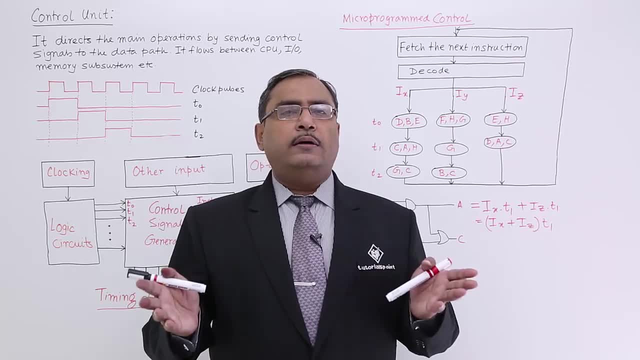 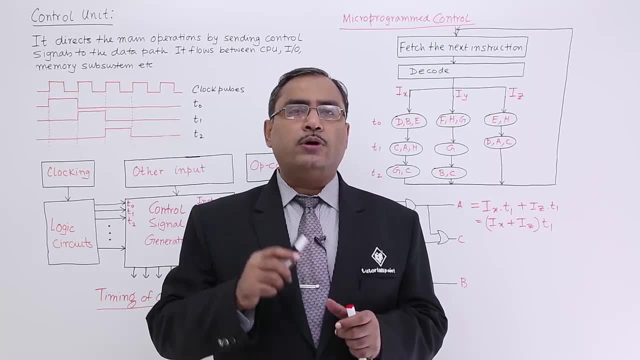 Control signals to select one device, whether say, take the example of memory After selecting a certain memory location through the address bus and the address decoder hardware. Now what can be done with the memory location? Should I go for read or should we go for memory? 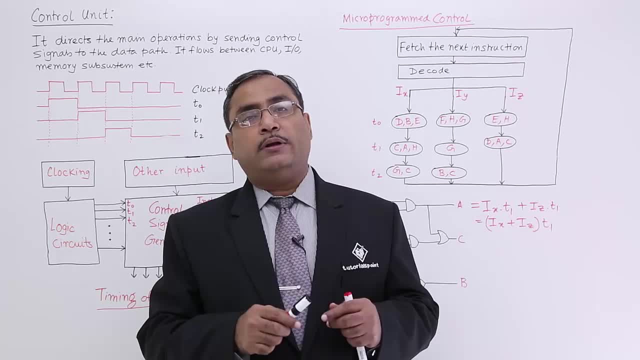 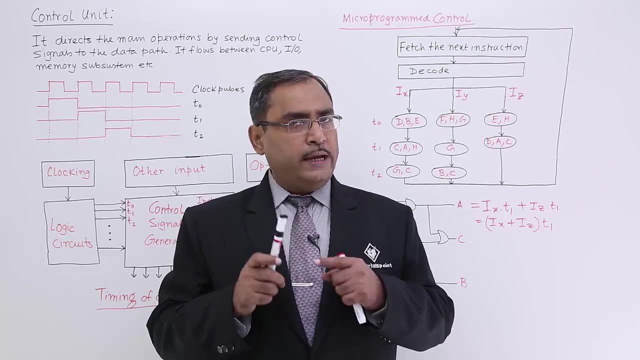 write. So control signal read and write will decide that one, whether I shall be going for memory read or memory write. Should I make one I O port for the input or for the output? So that will be decided by the control signal. Should I make this data?